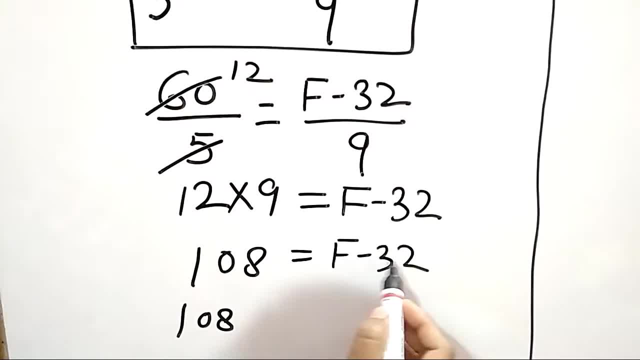 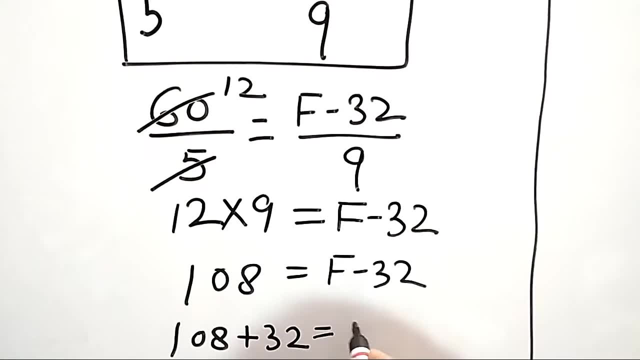 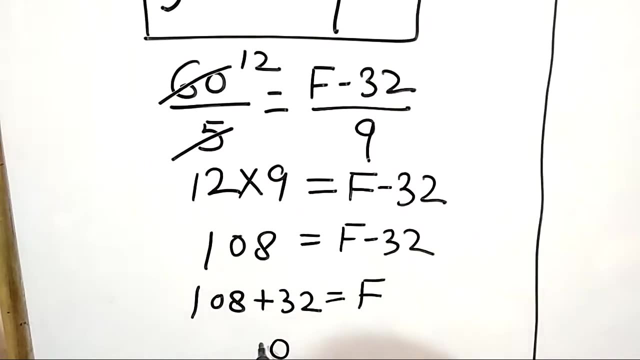 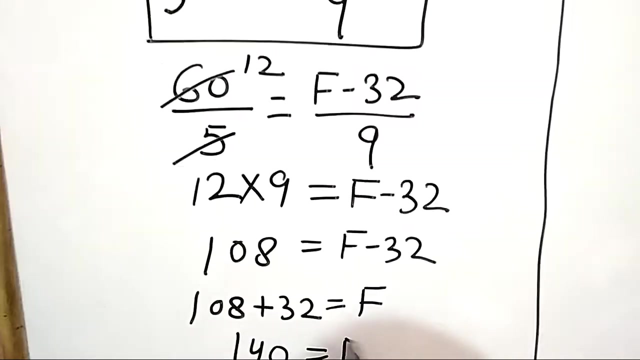 108.. When we will bring this 32 here, it will be plus 32,, which is here. minus 32 is equal to F. Now add this 8 to 10 and 4 and 1. 140.. So here we have find out value That. 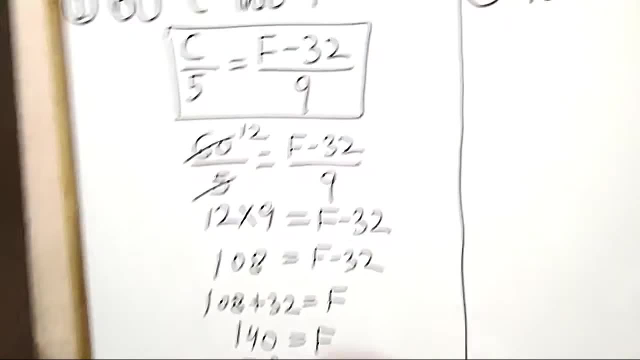 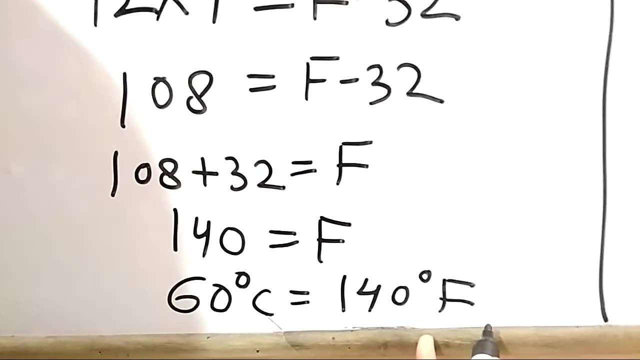 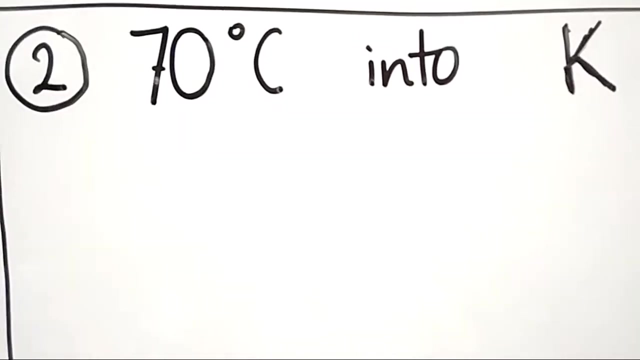 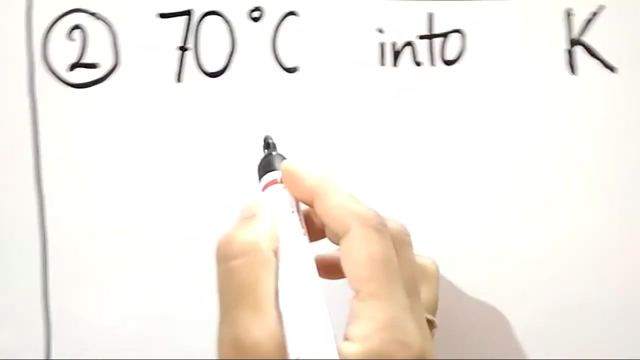 means 60 degrees. 20 degree Celsius is equal to 140 degree Fahrenheit, changed to Fallout 9.. Our next question is: convert 70 degrees Celsius into Kelvin. So convert this into Kelvin. We will take formula. this formula C is equal to K minus. to 70 degrees C. So power divided by 2 is equal to 10 to the over 1300 hertz. This appears 10 to 15 degrees, 6,, 0,, 12, and 1.. 4 times 10 to the over 3000 hertz. So we are turning onto. 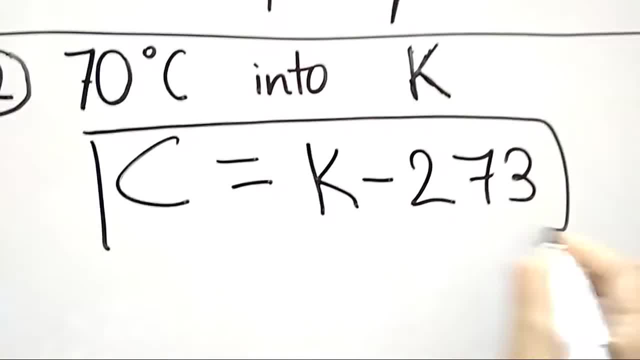 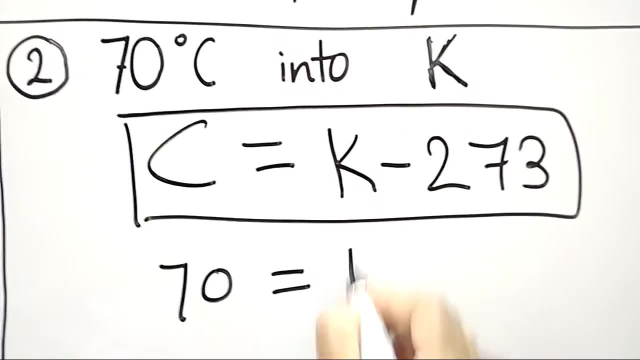 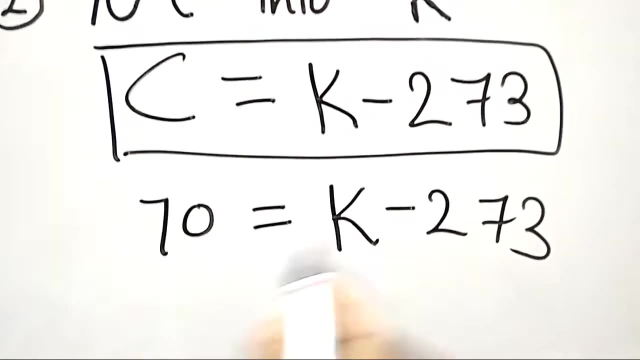 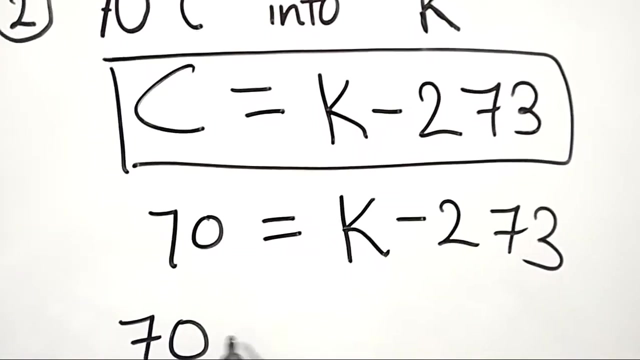 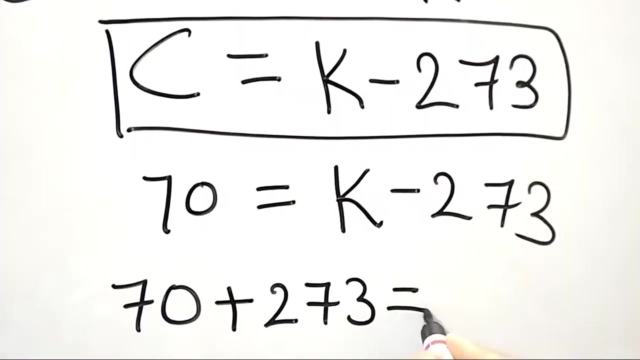 273. now put values, so 70 degree in the place of C, K, we have to find out, and minus 273, so we have to find out K. so we will bring minus 273 this side, left side, so it will be plus 273 because it is here, minus 2 is 273, it's equal to K. now, 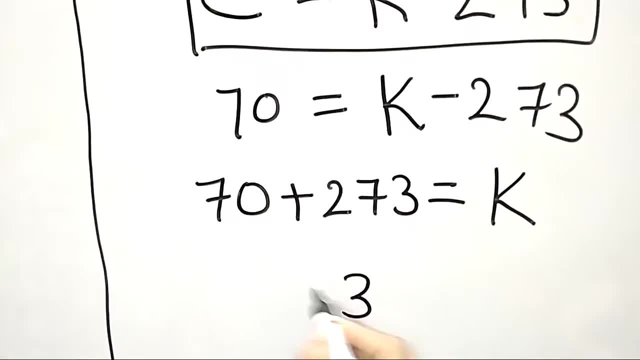 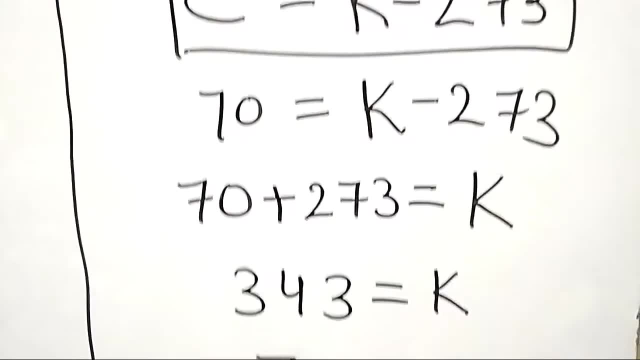 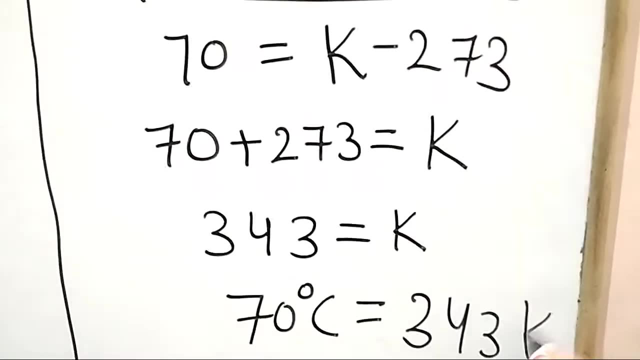 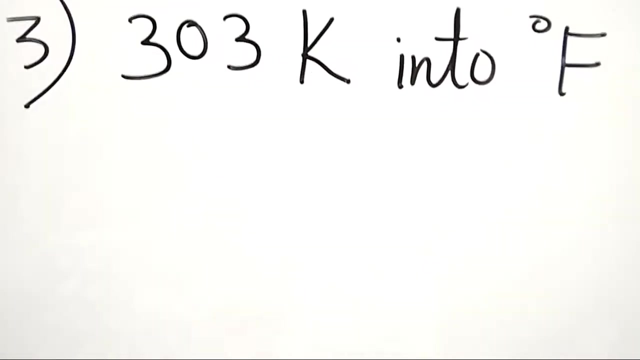 at 3, 7, 7, 14, 4 and 1, 3, 3, 43, it's equal to K. so we can say 70 degree Celsius is equal to 3, 43 Kelvin. question number two, three, is converter 303 Kelvin in two degree Fahrenheit. so to find out this: 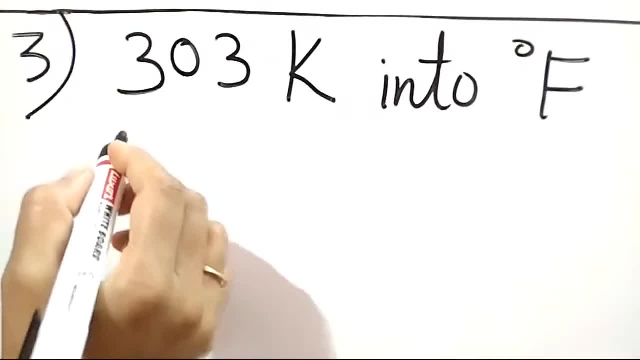 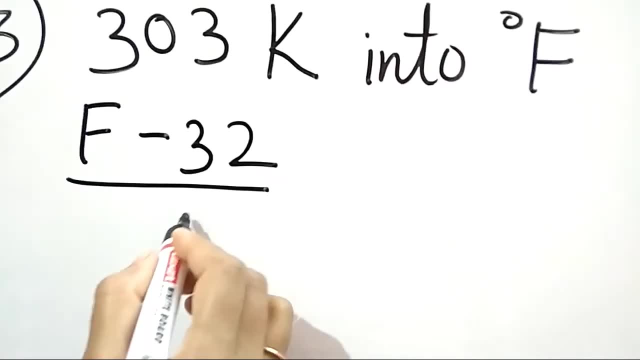 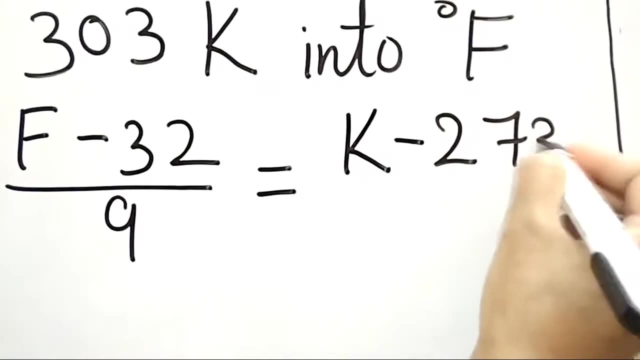 value. we will put this formula: F minus 32 upon 9 is equal to K minus 273 upon 5. so we have to find out this value. we will put this formula: F minus 32 upon 9 is equal to K minus 273 upon 5. 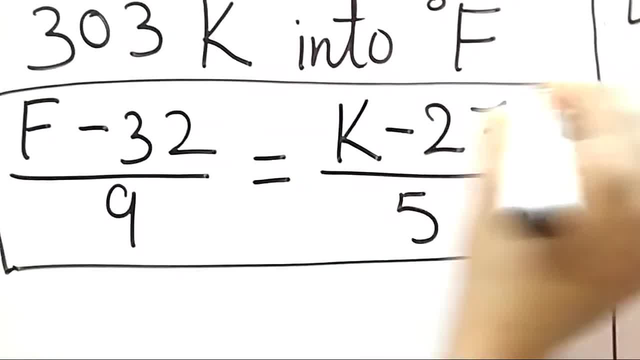 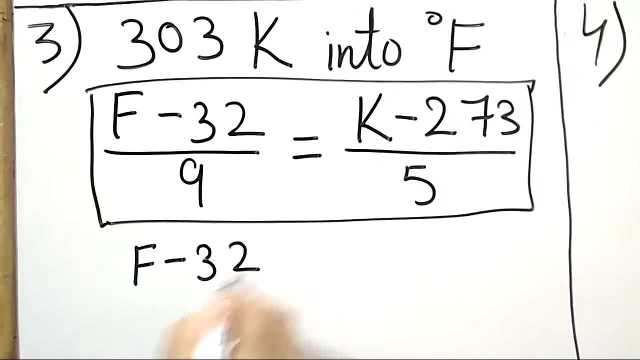 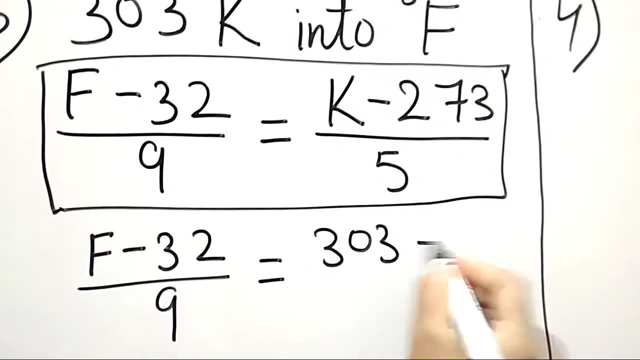 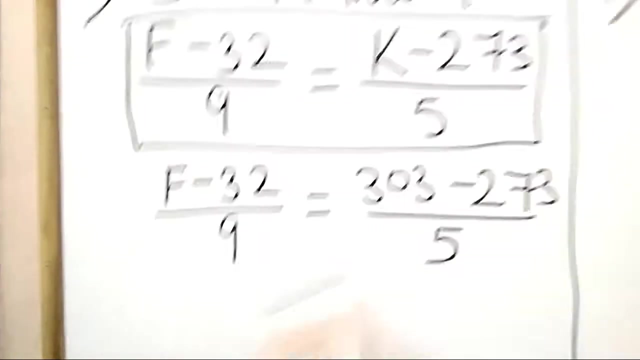 and put values in this formula. so here F, we have to find out. F minus 32 upon 9 is F. so here F, we have to find out. F minus 32 upon 9 is equal to K. it is given 303 minus 273 upon 5. first we will subtract it, so a minus 32 upon 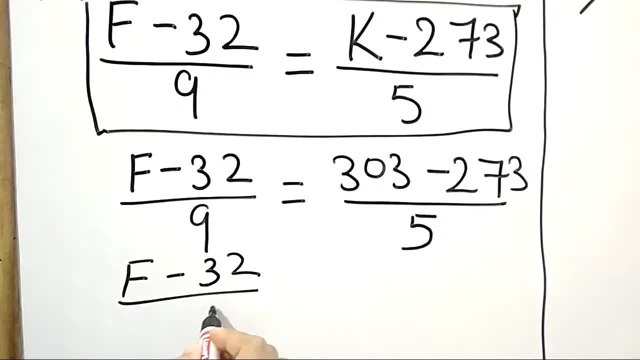 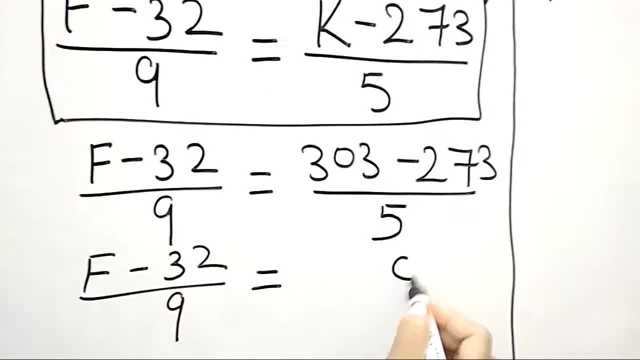 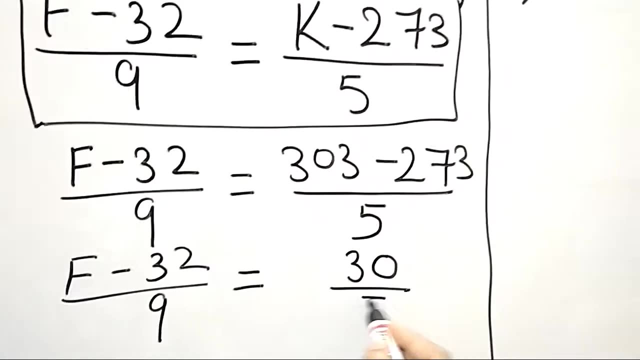 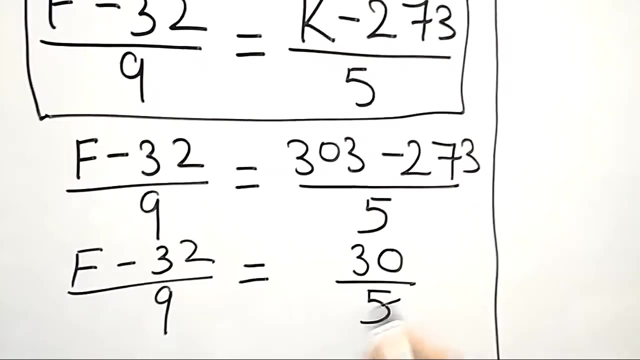 5, 9 is equal to 3 minus 3 is equal to 0, 10 minus 3 is equal to 3 and 2, 30, only 30 and 5. you can see it is visible with the visible. so now, divided 5, 6 up, 30 we. 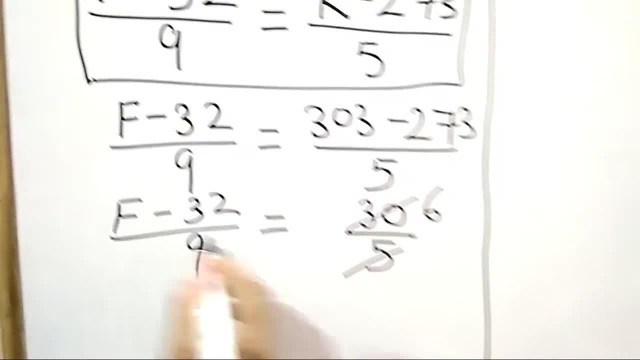 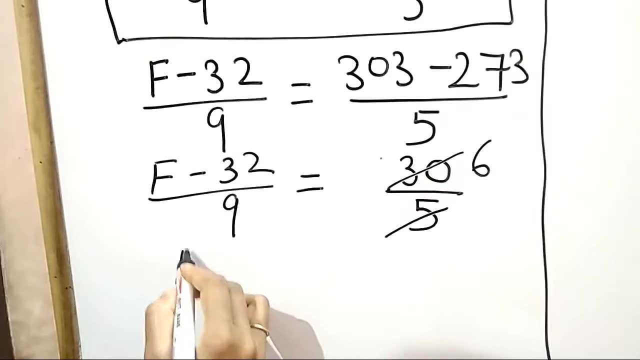 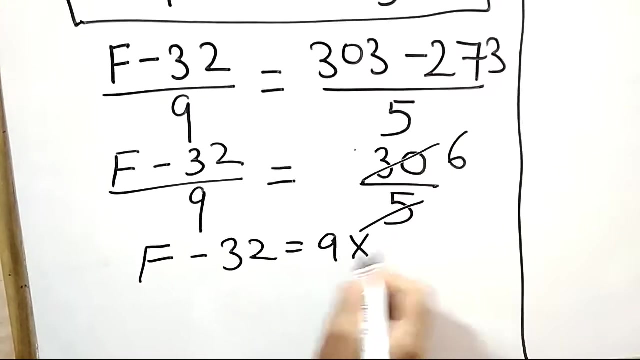 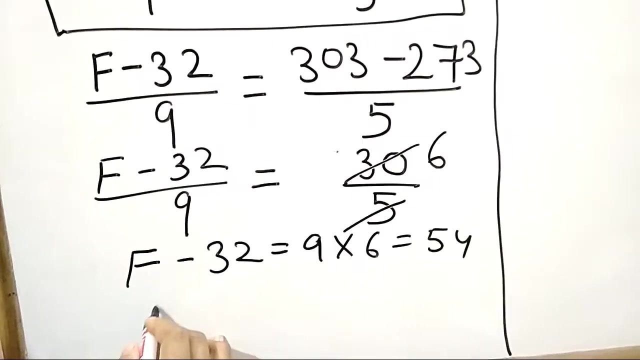 will get 6 here and we have to find out F. so we will cross multiply. so here it is: F minus 32 is equal to 9 into 6. that means we can say 54. we can write here only 54 and so find out F. we will put here F is equal to this minus 32 will. 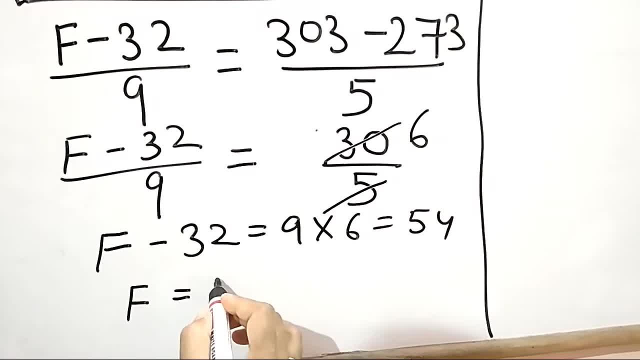 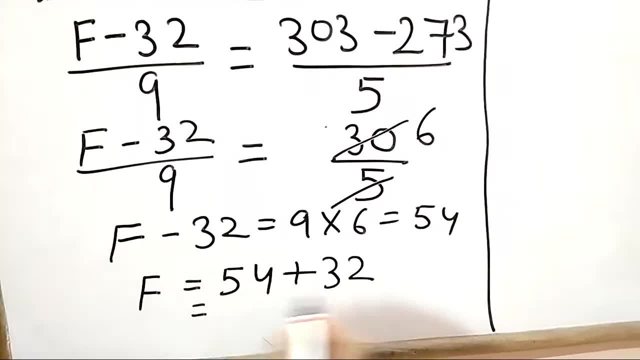 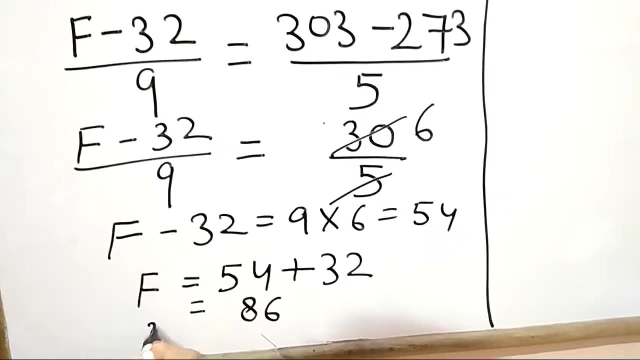 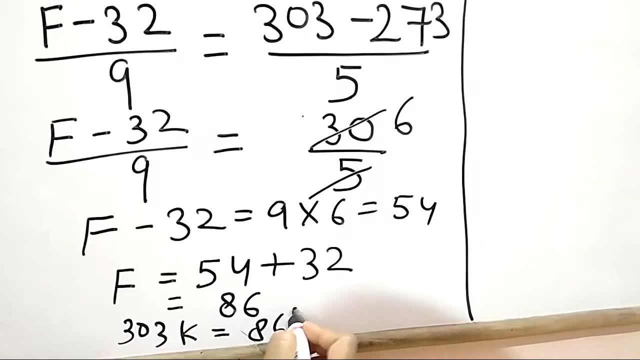 go this side, right hand side. so here we will write 54 plus 32, now at 4, 2, 6, 5, 3, 8, 86, so we can say 303 K is equal to 86 degree Fahrenheit. all we will go this side, right hand side. so here we will write 54 plus 32, now at 4, 2, 6, 5, 3, 8, 86, so we can say 303 K is equal to 86 degree Fahrenheit. 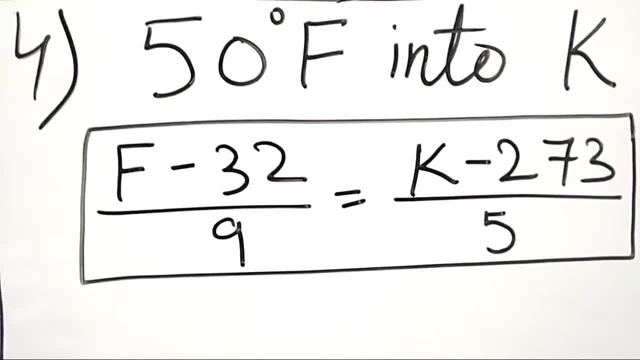 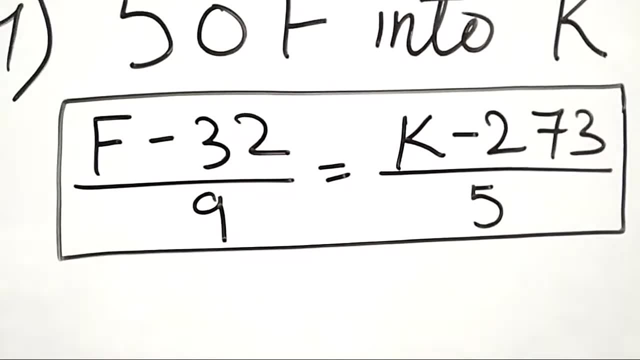 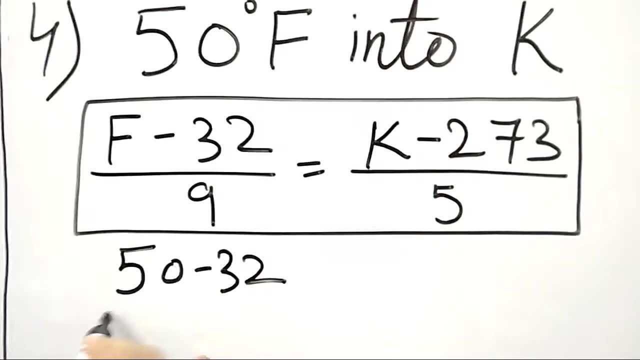 our fourth question is to convert 50 degree Fahrenheit into Kelvin. to solve this we will take same formula which have taken in earlier question. now, put values, F is equal to 50-32 upon 9 is equal to K. that is, we have to find out. 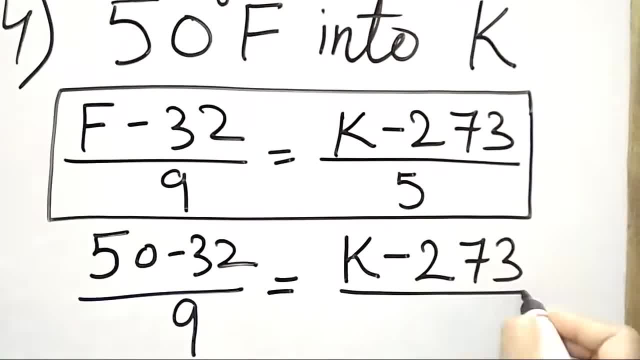 minus 273 upon 5. now subtract this value and we get K. we will take similar formula as we have taken in earlier question. now put values: F is equal to 50-32 upon 9 is equal to K. That is, we have to find out. minus 273 upon 5, now subtract this value.